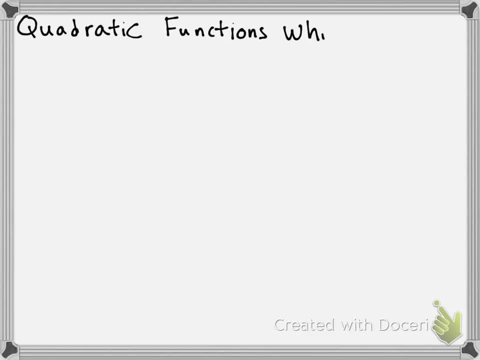 Okay. so what I'd like to talk to you guys about today are families of quadratic functions, So quadratic functions which share roots but have a different, a value. so it's a leading coefficient. they belong to a family, okay, So they have the same x-intercepts but they're 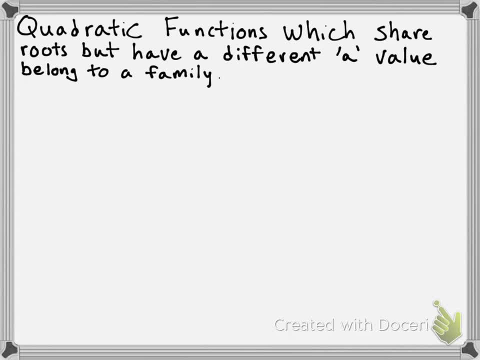 going to have a different leading coefficient and we say that they belong to a family. So let's take a look at the kind of question you might get which involve families of quadratic equations. So, for example, what we're going to do here is we're going to determine the 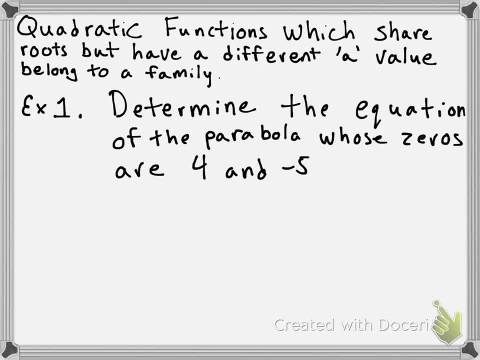 equation of the parabola whose zeros are 4 and negative 5,. okay, Now that alone, or those alone? those two zeros are not enough to determine the full equation of this particular parabola. We're going to need a little bit more information. It will be enough to determine. 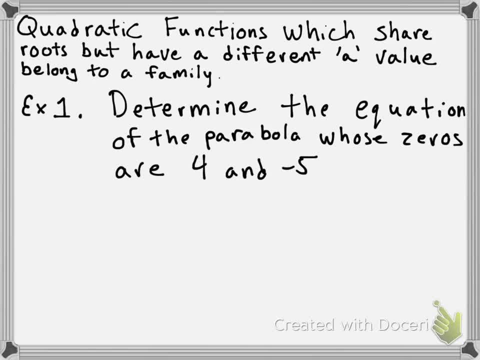 the family that it belongs to. okay, But it won't be enough to determine the a value. It will not be enough to determine the leading coefficient. So we're going to need one more bit of information, and that bit of information is going to be which point it passes through. 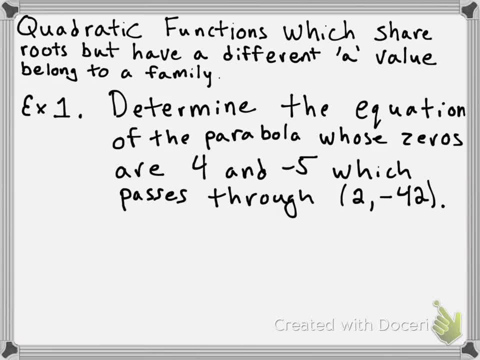 Okay, Specifically, this is going to be the quadratic equation that belongs to the family of parabolas, whose zeros are 4 and negative 5, which passes through the point 2, negative 42. That will be enough to specify a specific parabola. okay, So what we're going to do to start this. 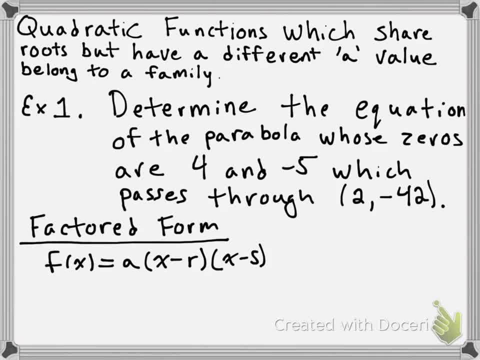 is we're going to deal with factored form Now. the reason we're dealing with factored form here is because we have the zeros, And factored form is the easiest way of writing a parabola that deals with the zeros. We can tell exactly where the zeros are and where. 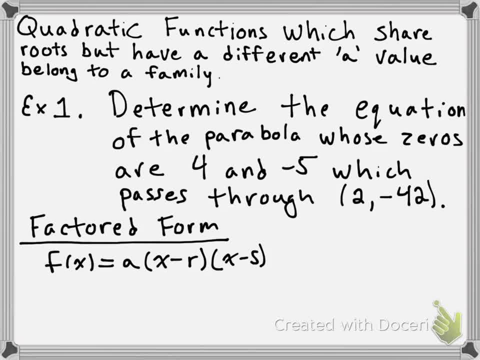 those zeros are going to go. So, specifically, we know that they're going to go in for r right here and s right here, okay, So we're going to be making the substitutions for those, okay. So when we make those substitutions, we end up getting: f of x is equal to a times. 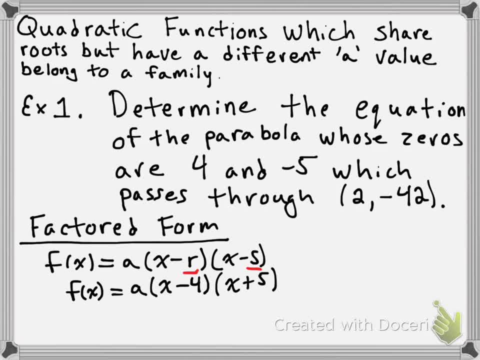 x minus 4 times x plus 5,. okay, Now this is enough to define the specific family. So that is the equation that defines the family of quadratic functions, But of course, in this question we're going to be looking for the specific parabola that passes through a point. So what?